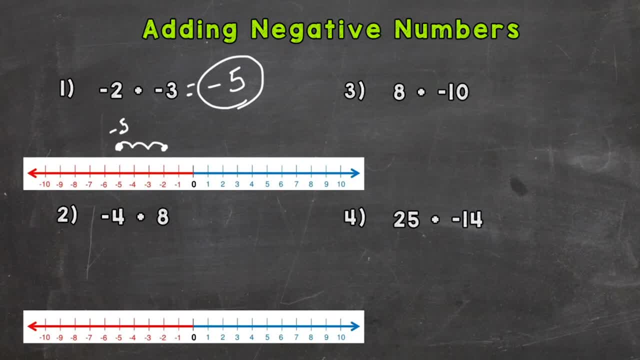 we end up at negative 5.. So let's take a look at number 2.. We have a negative 4.. We start here at negative 4, and we're adding a positive. So instead of going to the left this time, we're going to go to the right. We're going to go the. 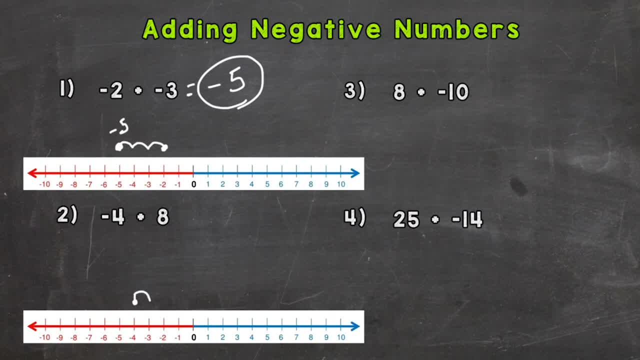 positive way, eight jumps: 1,, 2,, 3,, 4,, 5,, 6,, 7,, 8.. And we end up on positive 4.. So if we start at negative 4, and we add 8,, we'll end on 4,, which is our answer. So we're going to go to the left. this: 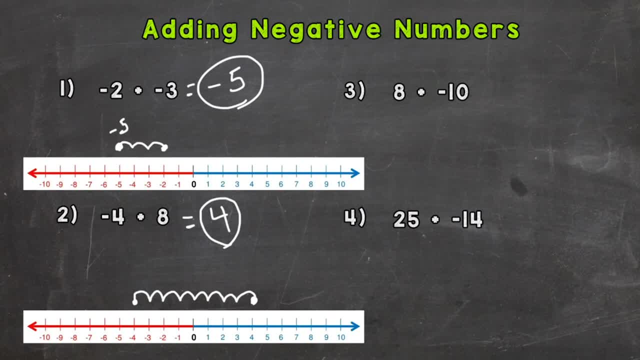 time, which is our answer. And if you think about it, let's think: if we had a temperature of negative 4, and the temperature went up 8 degrees, the temperature would now be a positive 4.. So let's take a look at number 3. We start with a positive 8, and we add a negative 10,, which is 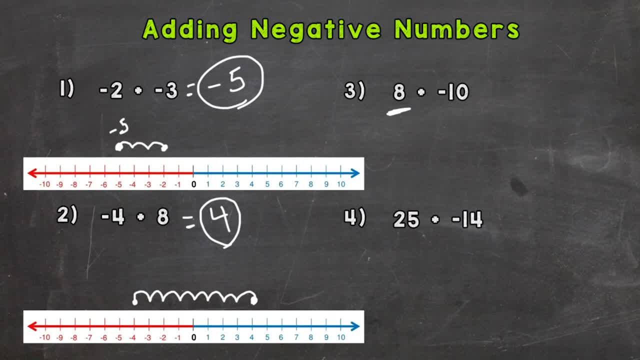 the same thing as subtracting 10.. We're going down 10.. So let's start at 8, and we're adding again 10.. So we're going to go to the left. 10 jumps: 1,, 2,, 3,, 4,, 5,, 6,, 7,, 8,, 9,, 10.. And we end up here. 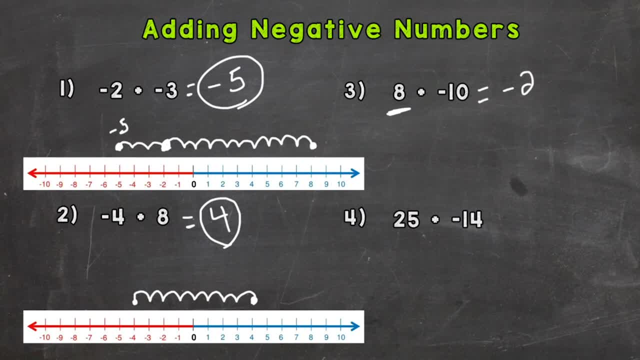 at negative 2.. We went below 0. And if you think about it, if you did 8 minus 8, you'd end up at 0. But since it's adding that negative 10, we're going to go to the left 10 jumps And we're going. 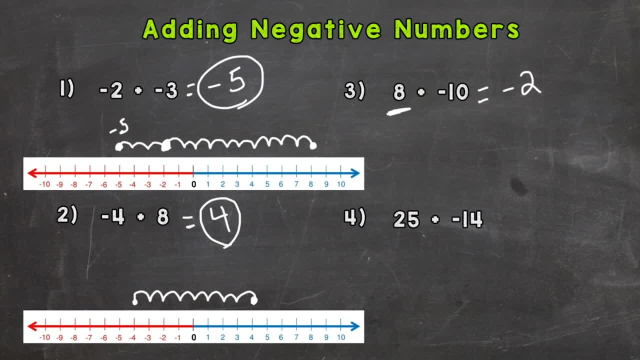 to add another negative 10.. We go 2 more below 0. So we end up at negative 2.. This problem is pretty much 8 minus 10.. Okay, and we go below 0. Again, we hit negative 2.. So let's take a look at number. 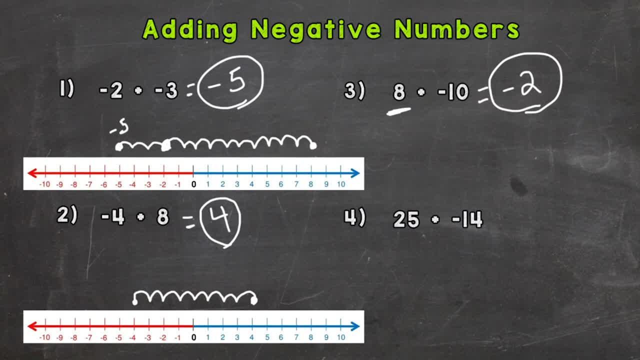 4. We start at 25, and we're adding a negative 14,, which is pretty much doing 25 minus 14, because we're going the opposite way. We're going to go to the left 10 jumps And we're going to